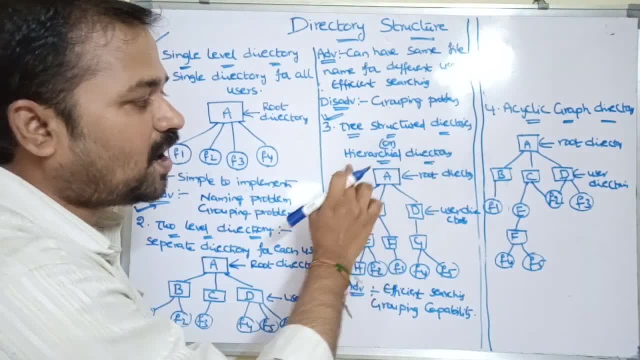 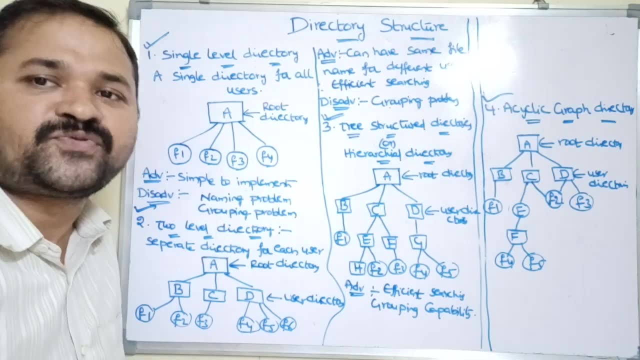 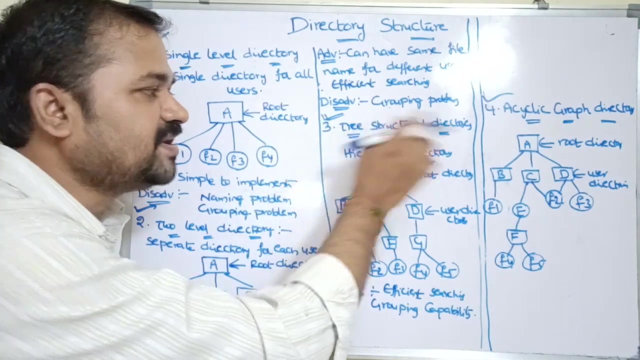 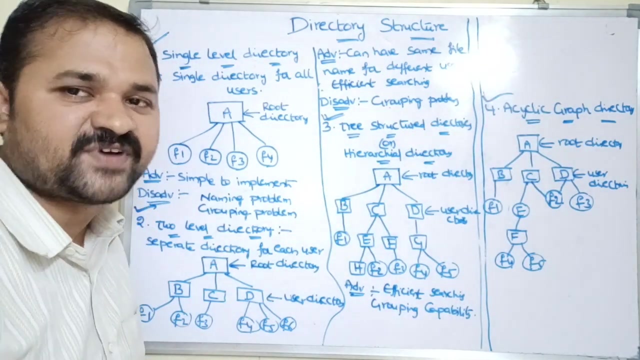 Third one tree structured directories or hierarchical directory. Fourth one acyclic graph directory. So mainly there are four types of directory structures are available: Single level directory. two level directory. third one tree structured directory or hierarchical directory. Fourth one acyclic graph directory. So let's see all these structures one by one. So first, one single level directory. 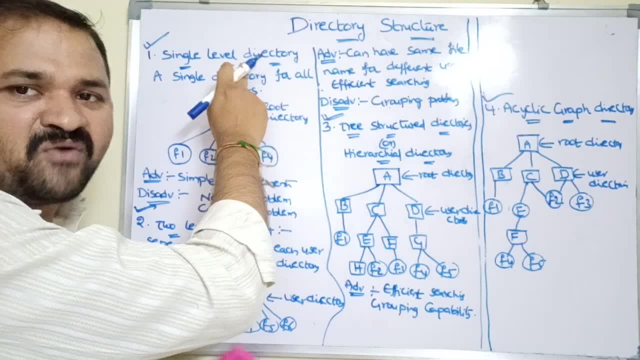 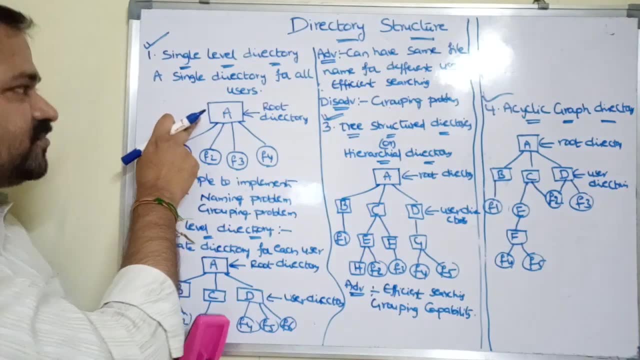 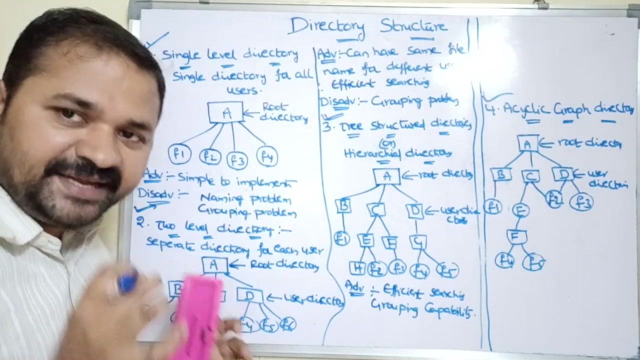 So the name itself specifies the meaning. we can have only one directory that is at the top level, level 0. so this is the directory that we are using here, so a single directory for all the users. so all the users in the system needs to create the file in in this directory only, okay, so that's why it. 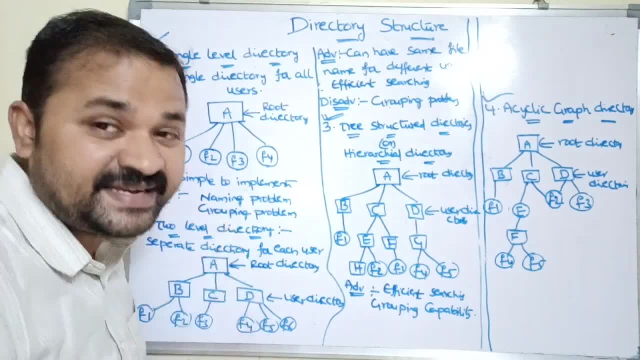 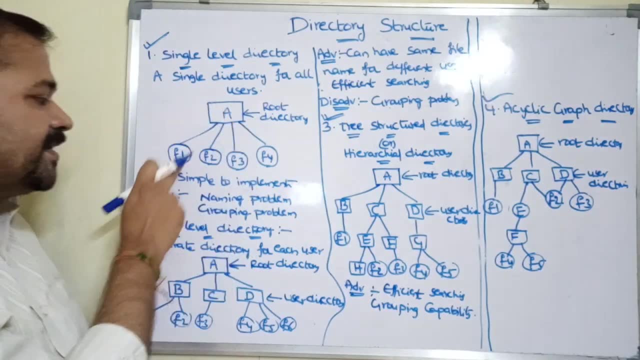 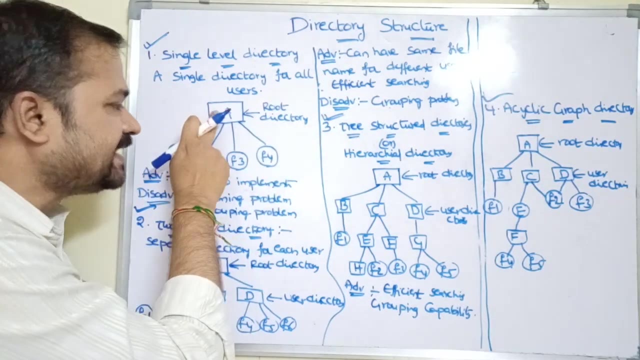 is known as single level directory, so we can have only one directory here, the top level. okay, here, in order to represent the directory, we are using a file, whereas in order to represent the file, we are using a circuit. so here, what is the directory? here a is the directory. we can call this directory. 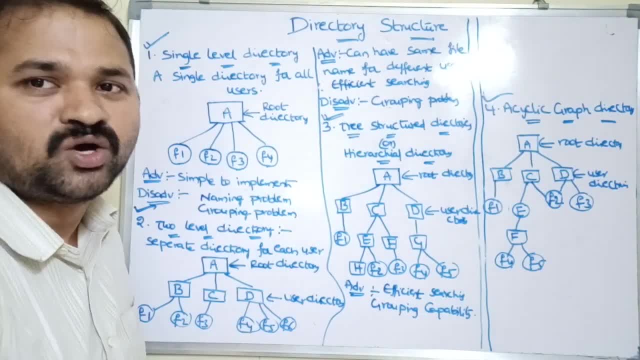 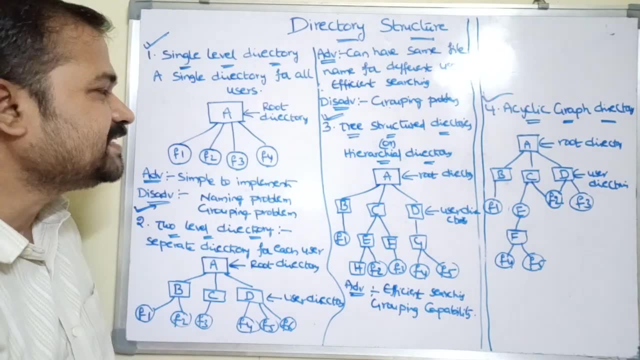 as root directory, because the topmost directory is known as a root node. so this is do directory. so this directory contains four files. you have one, you have two, you have three. let's see the advantage of this approach. it is very, very simple to implement this approach. why? because we need to. 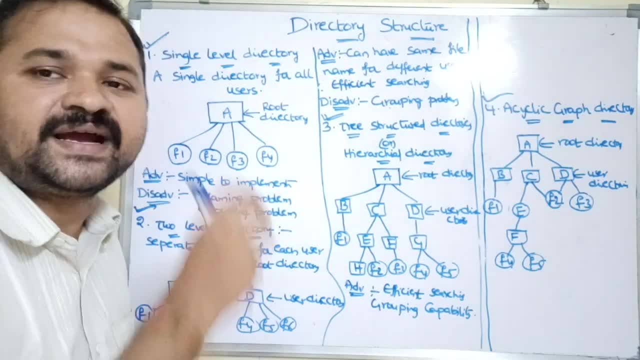 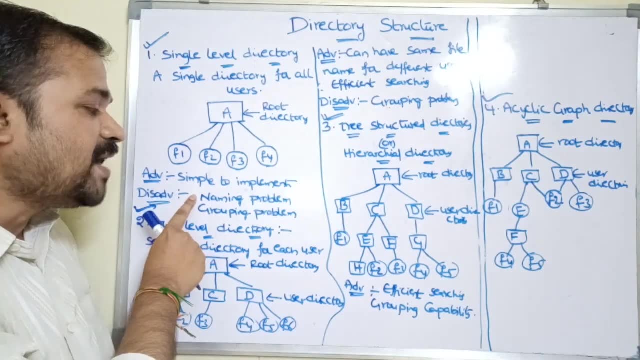 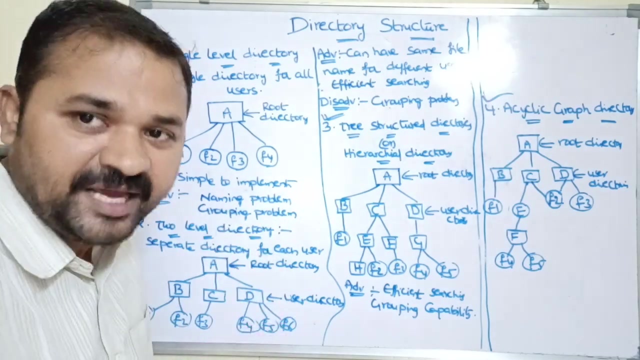 have only one directory and all the files needs to be stored in the directory only. so it is very, very simple to implement this approach. and let's see the drawbacks here. the first drawback is naming problem. so sometimes there may be a possibility that multiple users can give a same name for their files. so let 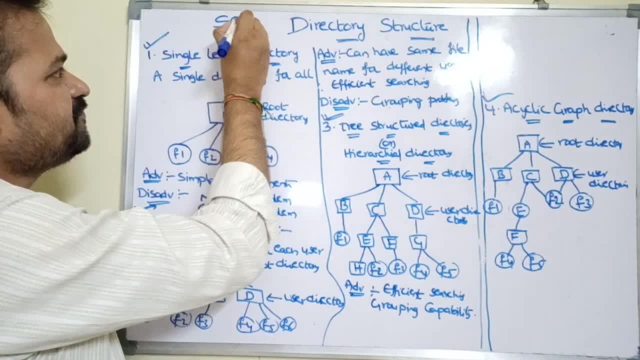 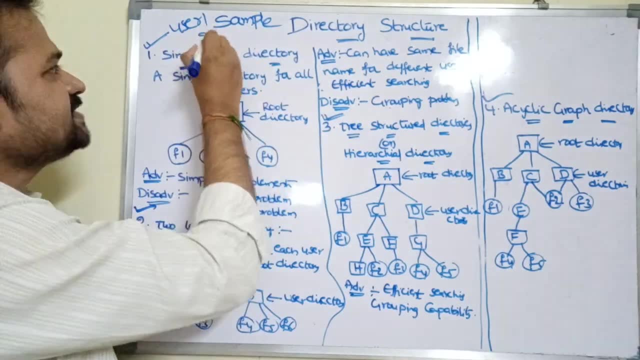 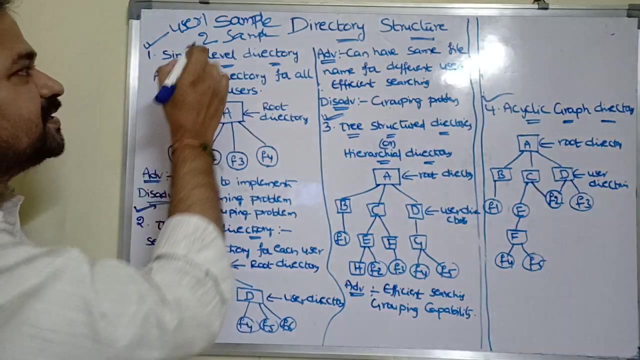 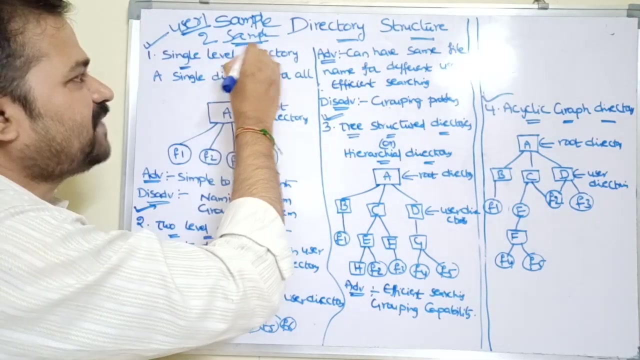 us assume that user one has given a name for the file as sample, so user one created a file with the name sample. let us assume that user two also created a file with the name sample. so then what will happen? user one file will be overwritten, so in place of that file, this sample content the sample file. 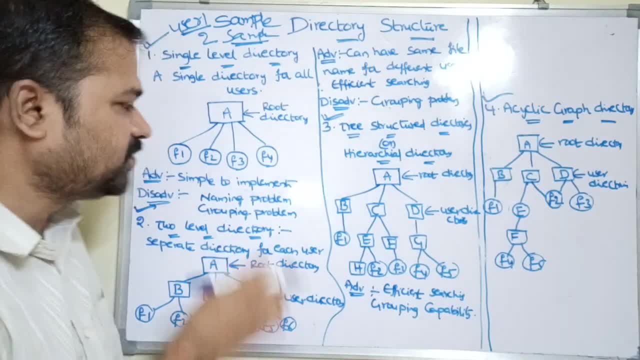 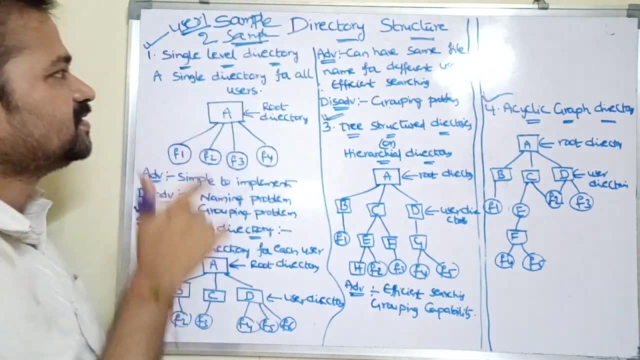 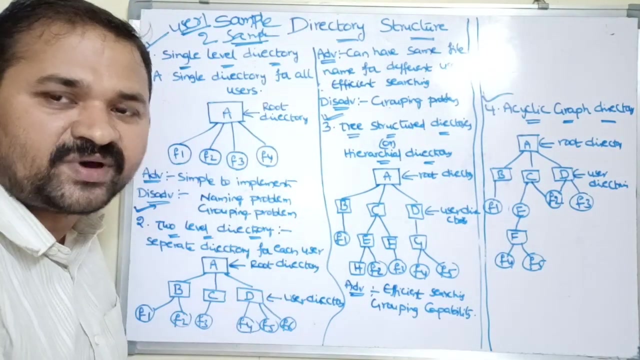 content will be stored. why? because here, how many directories are available? only one directory is available, so in that directory only we have to store the files. so user one created a file with sampling. so user two also created a file with sampling. so then what will happen here? user one sample file will be overwritten with user two sample file. so that is the first. 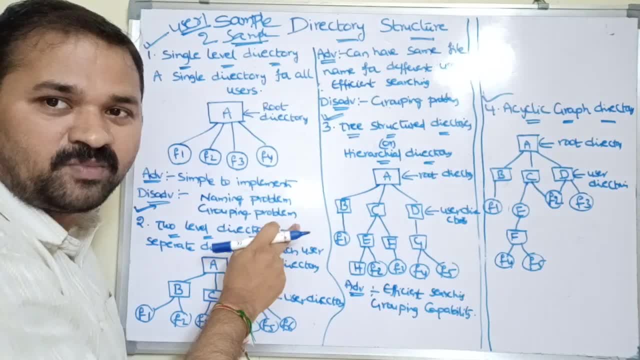 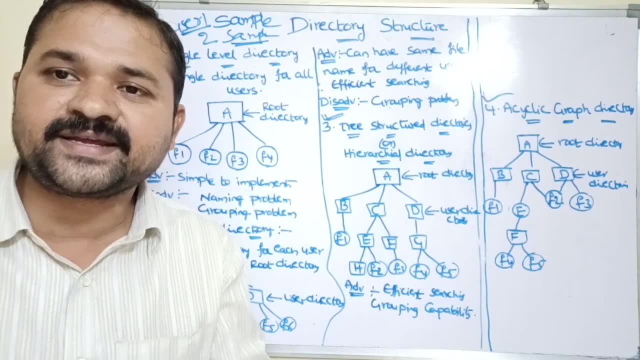 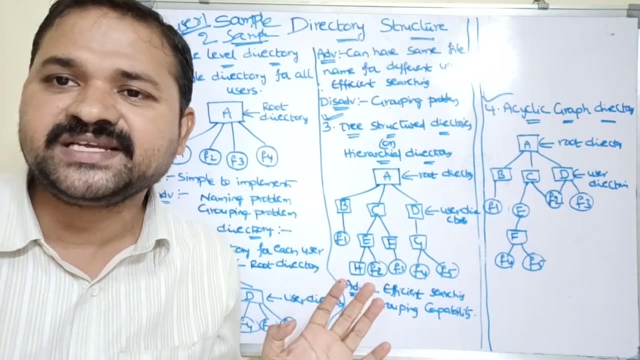 problem here: naming problem. and the second problem is grouping problem. let us assume that I want to store C files in a single directory, C++ files in another directory, Java files in another directory. but that is not possible here. here we can have only one directory. all the files needs to be. 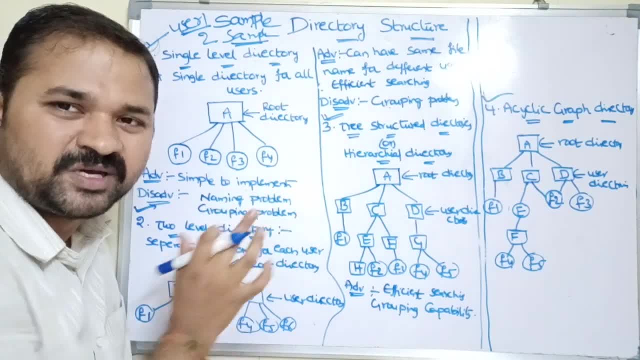 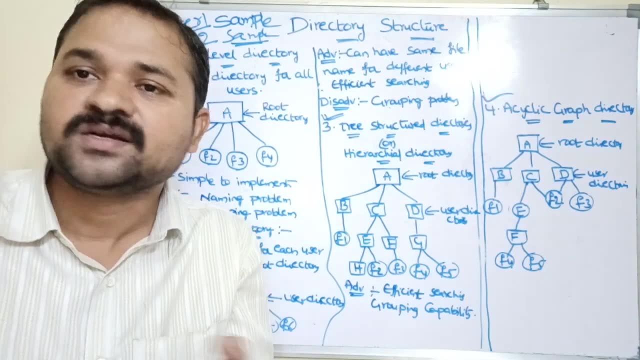 stored in the directory only. so this is the second problem, grouping problem. so it is not possible to group a collection of files in one directory and one more collection in the other directory. so likewise it is not possible here. so we can overcome these problems with the help of the second approach. 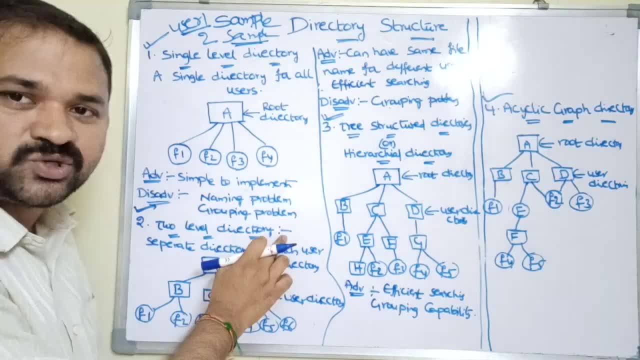 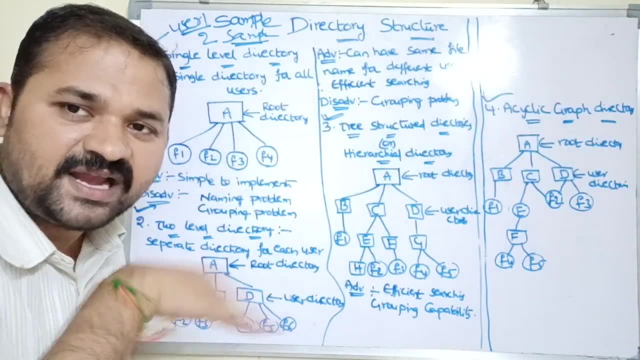 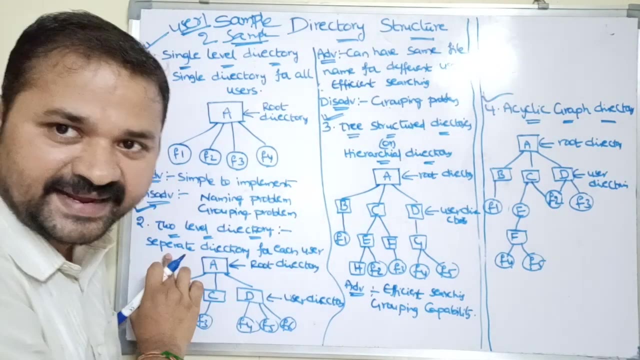 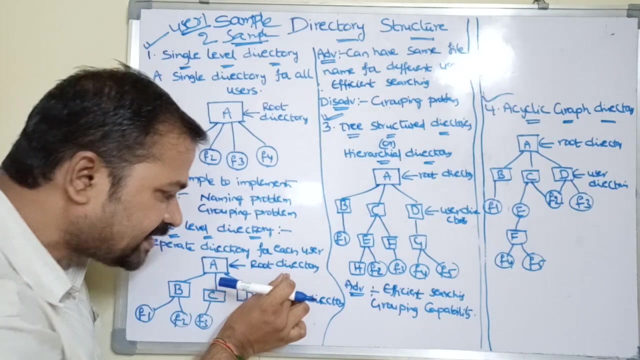 the second approach is two level directory. so the name itself specifies the meaning. here we have directories at two levels. so level 0 contains one directory, level 1 contains another. directories like that. so separate directory for each user, okay. separate directory for each user, okay. so in this example, capital A is nothing but our root directory. so inside the root directory we 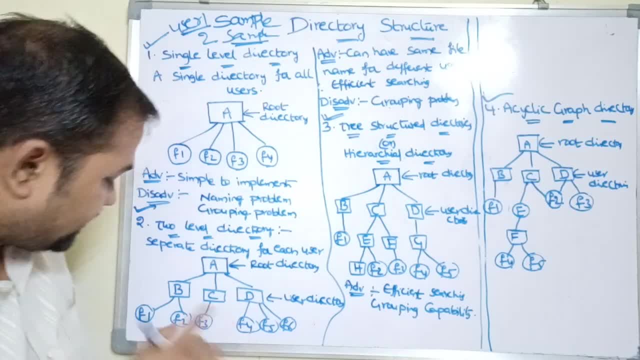 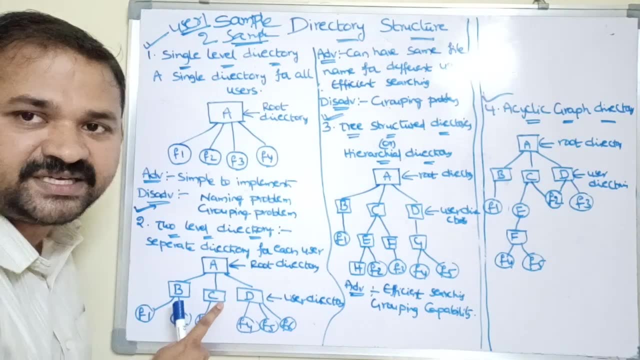 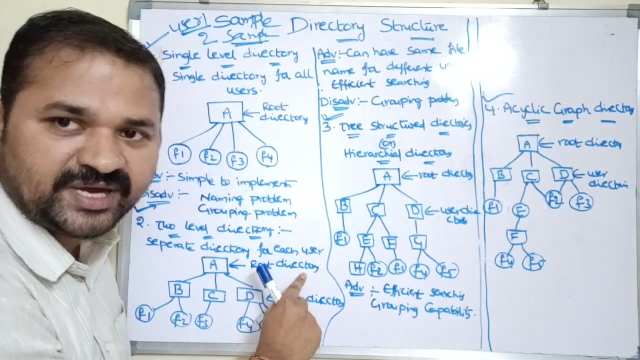 can create user directories. let us assume that there are four users here, so three users here. so user 1 created a directory called B. user 2 created a directory called C. user 3 created a directory called C. okay, so here we have directories at two levels. so level 0 contains two directory. 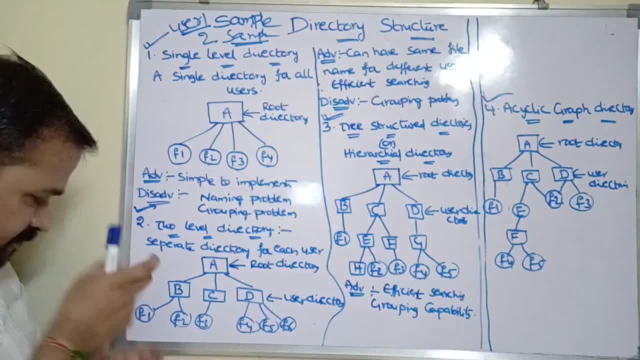 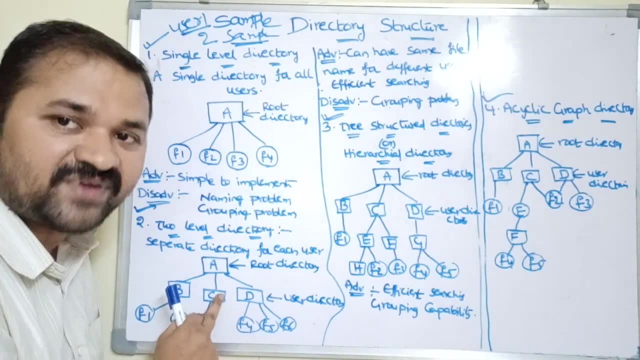 level one contains user directory. so now this B directory, files can be stored here. you have two or nothing but the files of B directory. you have three is nothing but the files of T directory. next you have four, you have five and you have six or nothing but the files of the D directory. so 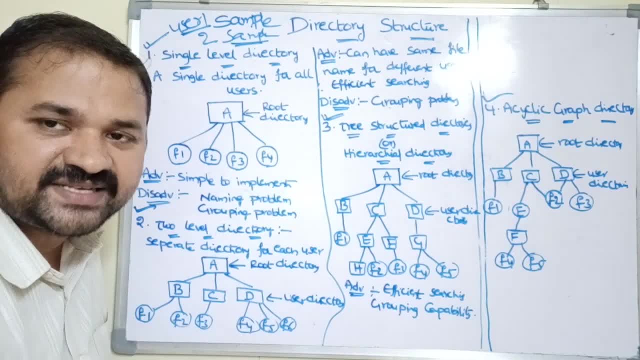 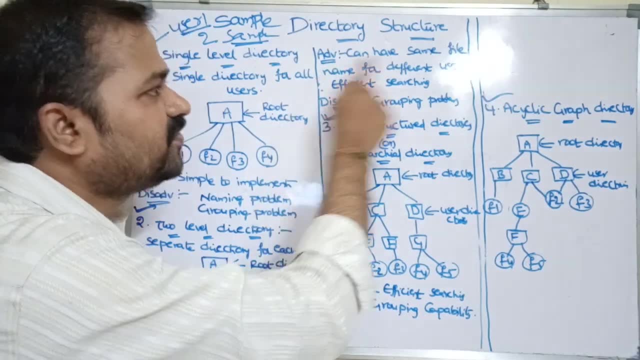 directories are represented with the help of square, whereas the files are represented with the help of circuit. now let's see the advantages here. the first advantage is can have the same file name for different users. why? because here we can have a separate directory for you for each user. 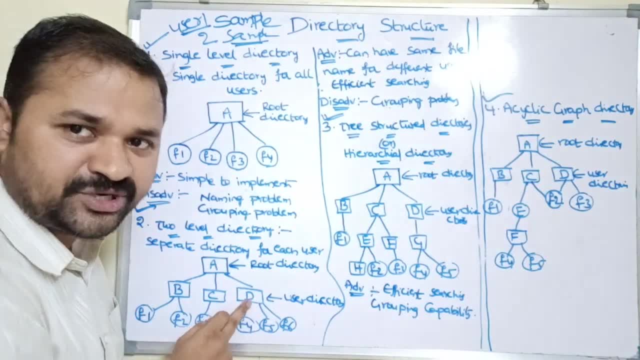 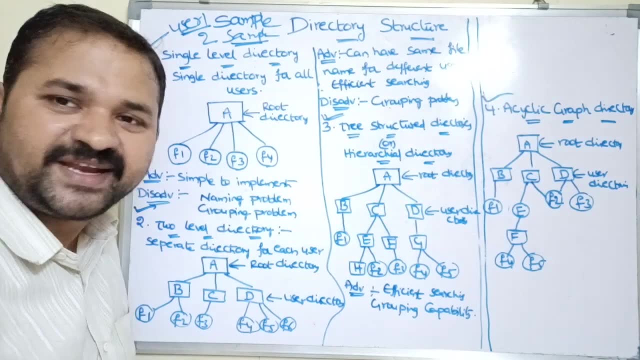 so user one may give a file name. you have one. user two can also give your file name as well: F1. user three can also give file name as F1. so there is no problem here. why? because for each user we can have a separate directory, so there is no naming. 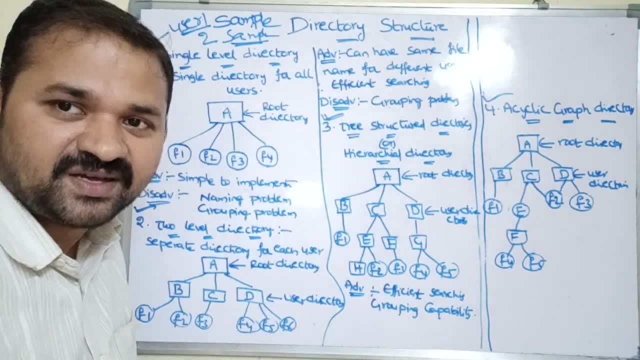 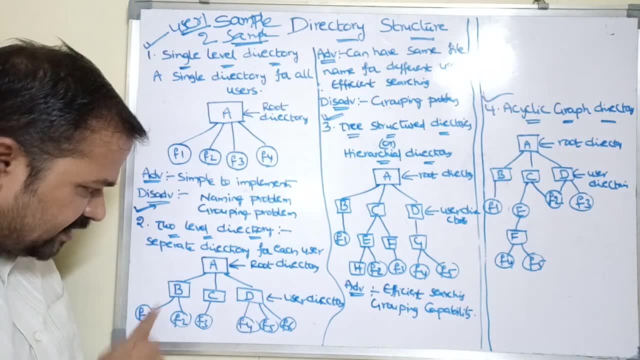 problem here. and one more advantage is efficient section. here we have efficient section. why? because we can have user directory also. so in order to search for the file F1, then we can search in A and B, so directly we can get F1 various if you take this one. 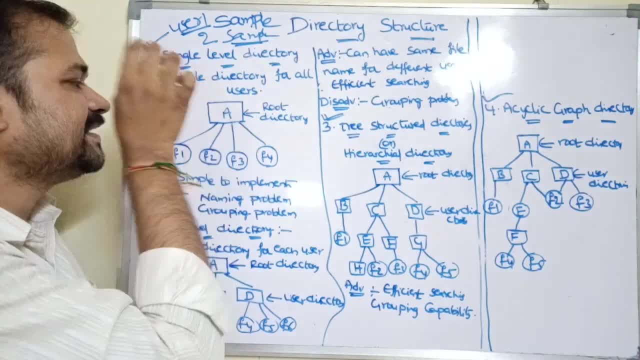 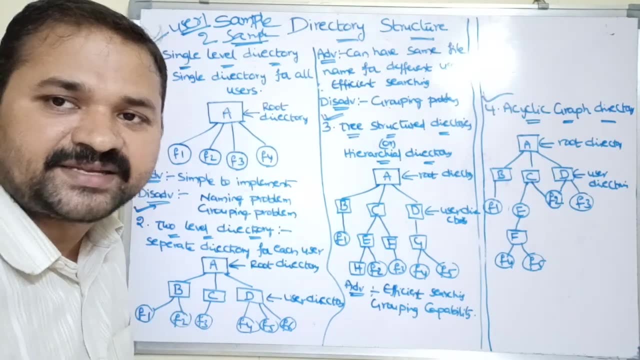 uh, single level directory, so all the files will be stored in a single directory so that for searching it will take more amount of time. various here for you chooser. we can have a separate directory so that for searching it will take less amount of time than if you compare with single level directory. 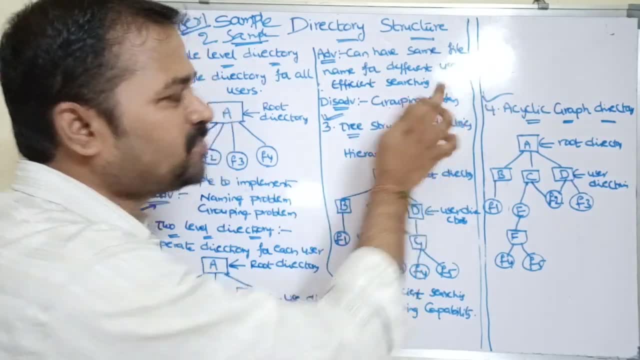 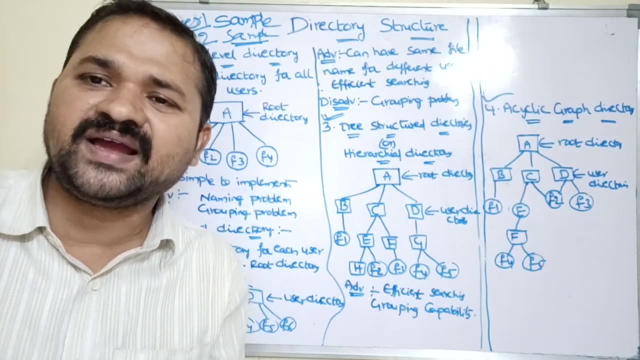 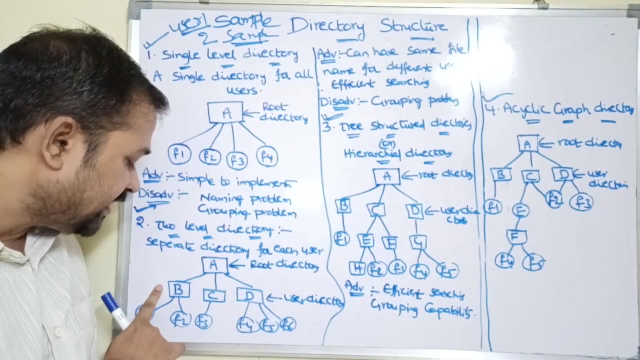 now let's see the drawbacks here. the drawback here is grouping problem. okay, let us assume that I want to store 100 files inside a directory. then we have to store all the 100 files in a single directory. I want to create sub directories inside a directory. I want to create two sub directories inside B, but 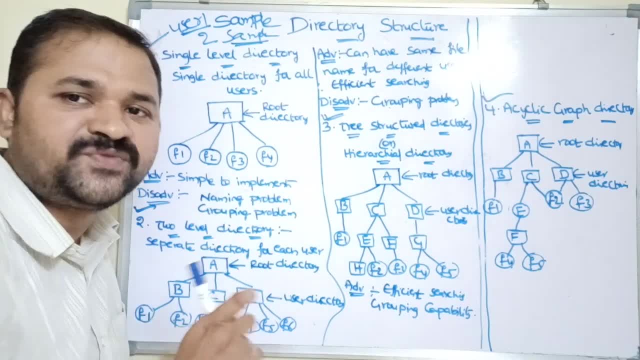 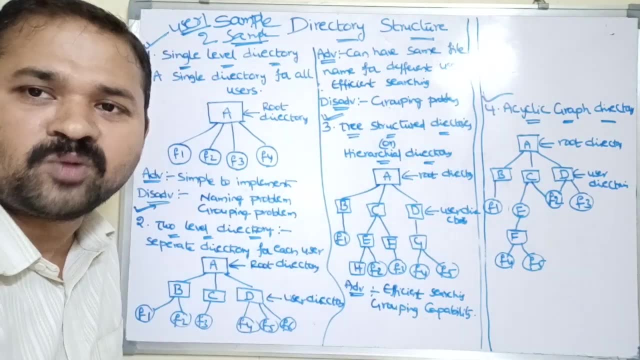 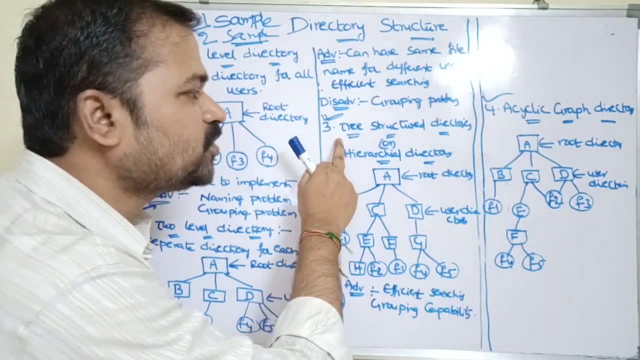 it is not possible here, okay. each user needs to maintain only one directory. sub directories are not possible to create here, okay. so that is another problem here. so grouping problem: it suffers with grouping problem. so in order to overcome this drawback, we can use as the third approach. the third approach is tree structure directories on hierarchical directory. so two level. 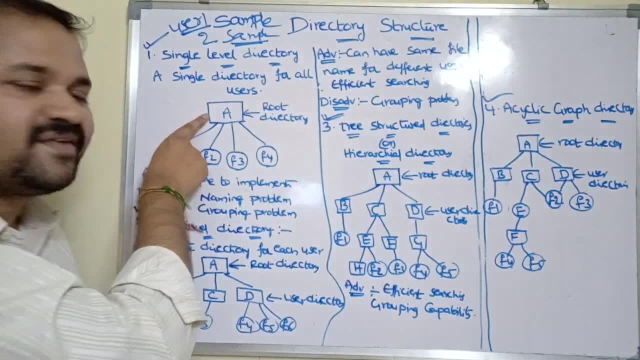 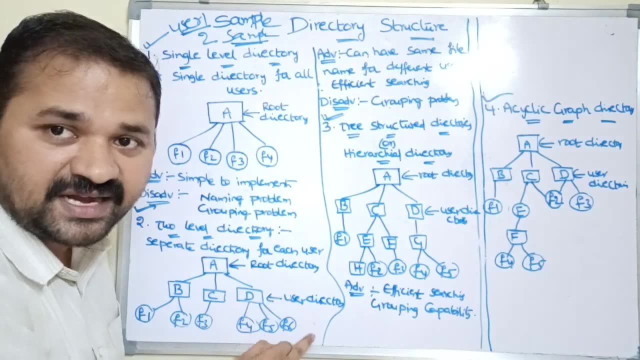 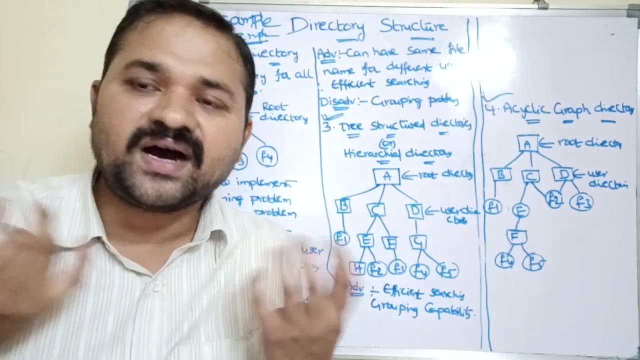 single level means we can have only one level, so in that level only we can have directory. so two level means we can have directories at two levels. so level zero is nothing but two directory. level one is nothing but user directory, whereas tree structure directory or hierarchical directory means we can have a. 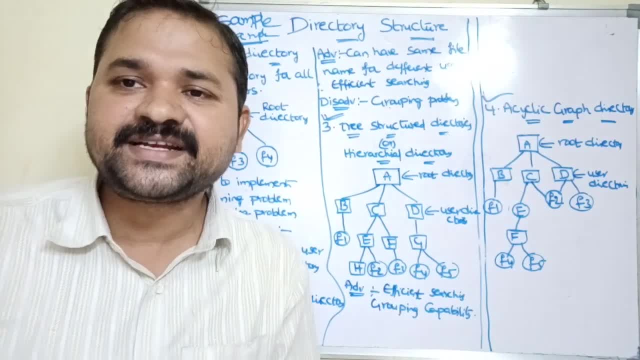 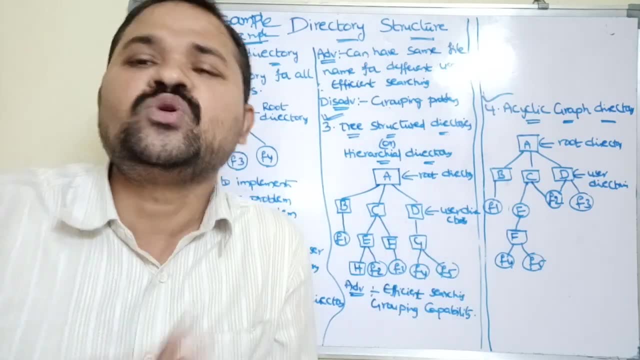 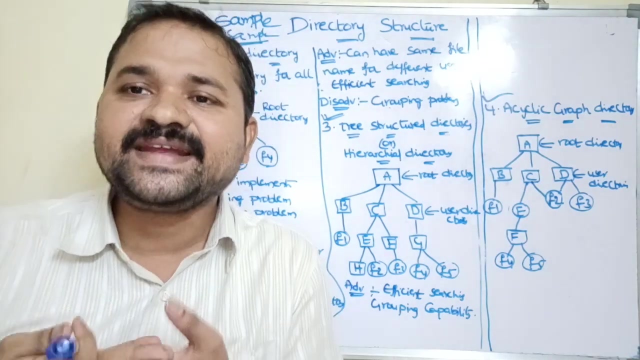 directory set different types of levels. so we know what is a tree. so tree means a collection of nodes, so we can create the nodes in different levels. so here we can have more than two levels, so we can have three levels or four levels, 50 levels or 100 levels or 200 levels or 1 lakh levels, so we can create any number of directories. 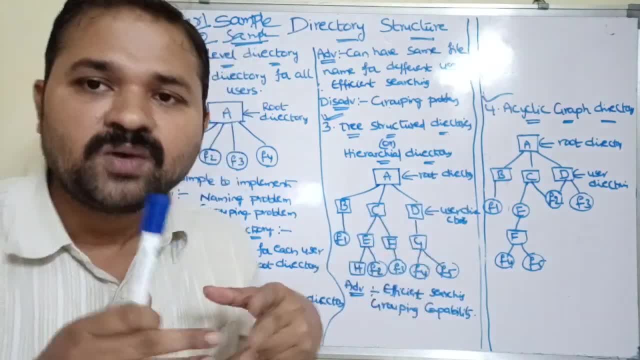 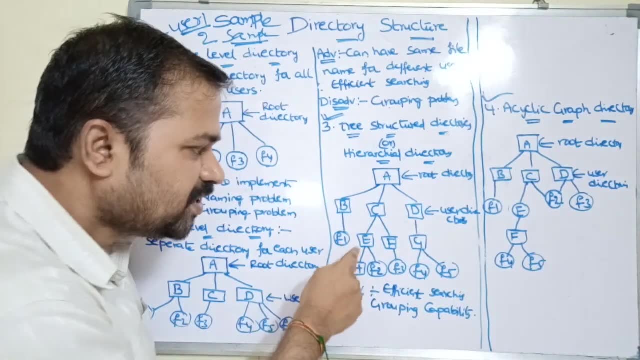 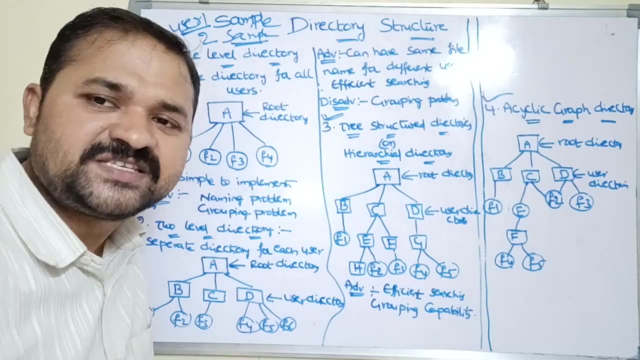 as we want, but here the directories should be at more than two levels. so what is level 0 here? root directory. level 1: user directories. next level 2: we can create sub directories again. level 3: we can create sub directories again. level 4: we can create sub directories. so likewise we can create. 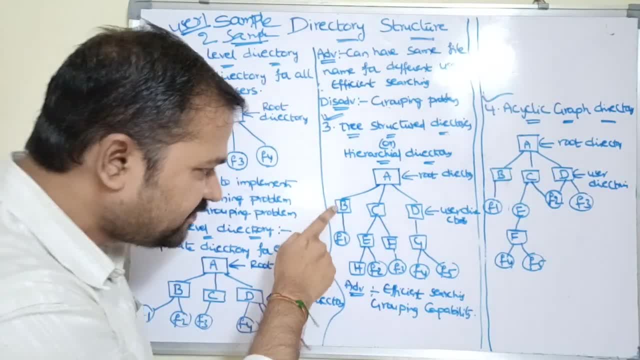 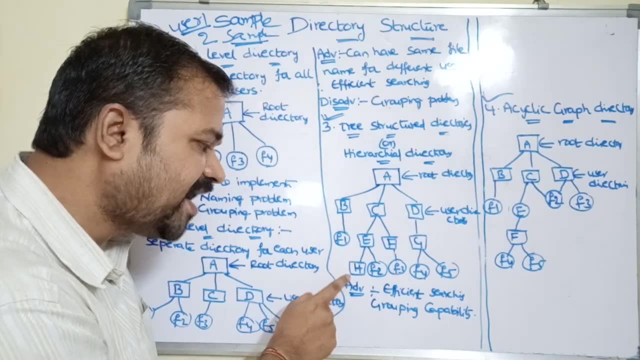 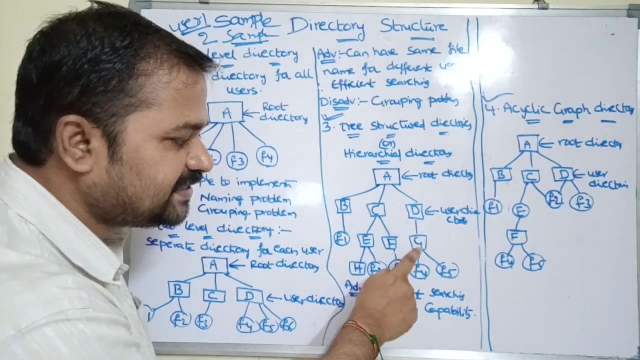 n number of sub directories. okay, so here in b directory we can have f1 file. in c we created two sub directories, e and f. so e contains again in e. we have a sub directory called h and we have saved f2 in e. next f directory contains f3, 5, z directory contains f4, f5, so likewise we can. 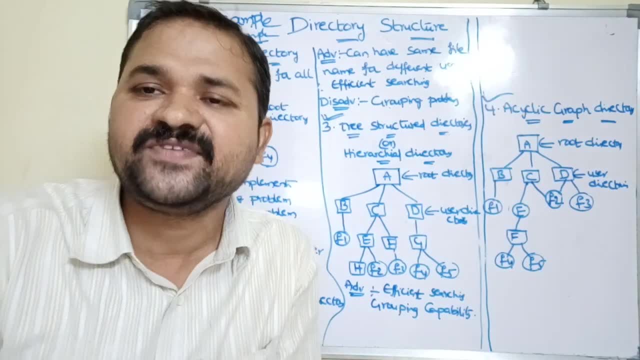 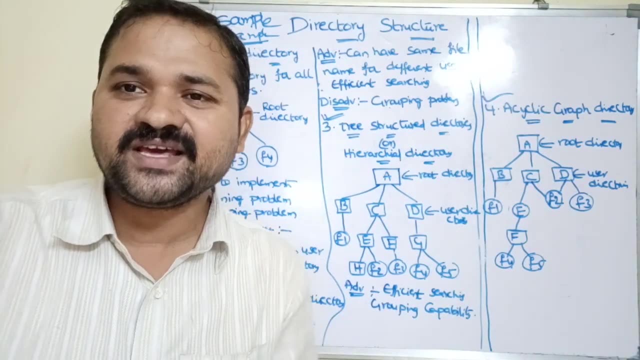 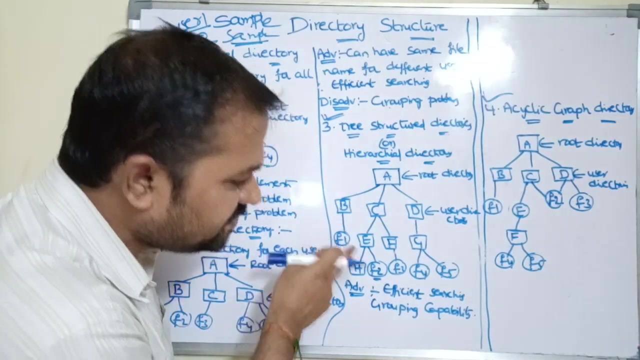 create n number of sub directories and in those directories we can store a large number of files. so the major advantage of this approach is efficiency. why? because here we can have a separate sub directories. let us assume that we want to access f2. then with the help of a, c, e, we can access f2. okay, so efficient setting it performs. 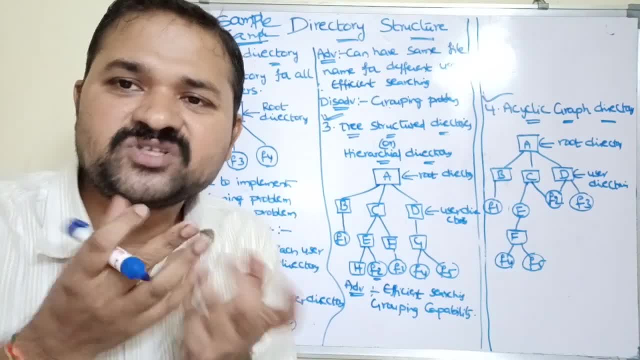 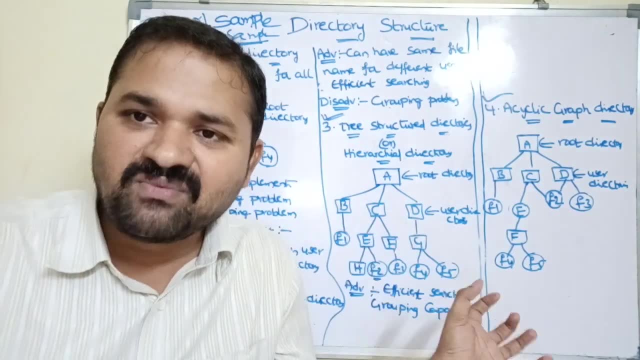 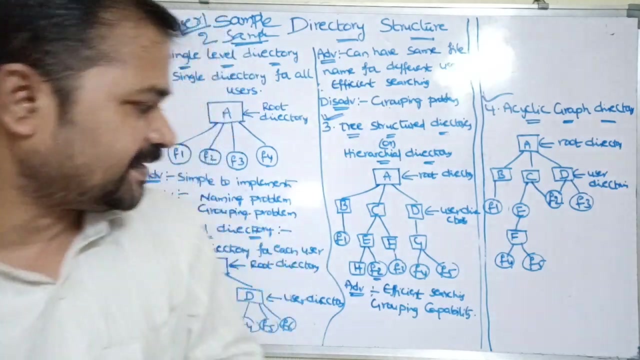 why? because too many sub directories are there, so with the help of those directories we can search for the file in efficient manner. and one more advantage here is grouping capability. here we have grouping capability. why? because we can have too many sub directories, so in those directories we can store n number of files. okay. 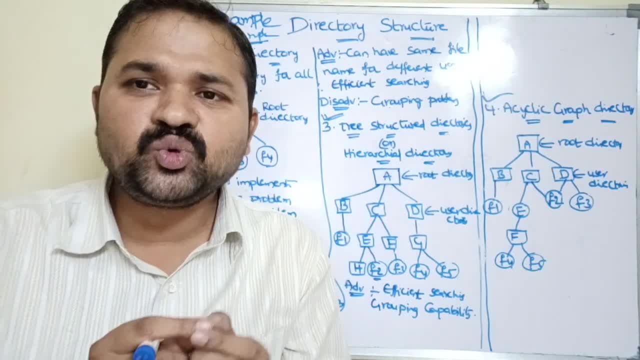 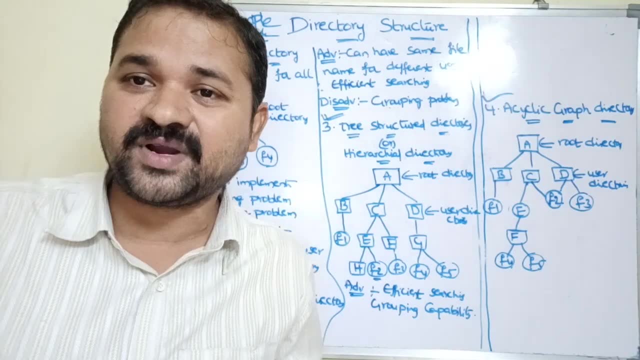 but here the problem with this approach is: if you want to share a file among different directories, then it is not possible. if you shared like that, then a cycle will be formed, but a tree doesn't contains any cycle, whereas a graph contains a cycle. okay, so you know to work on this problem. 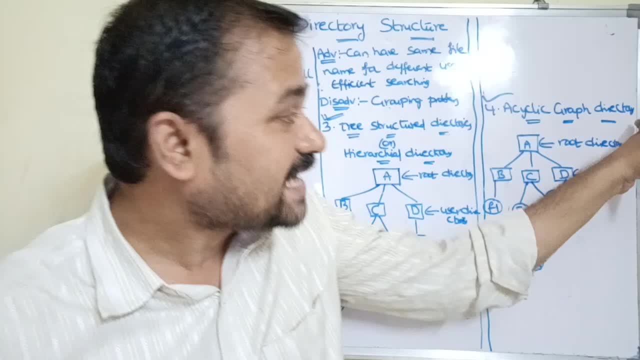 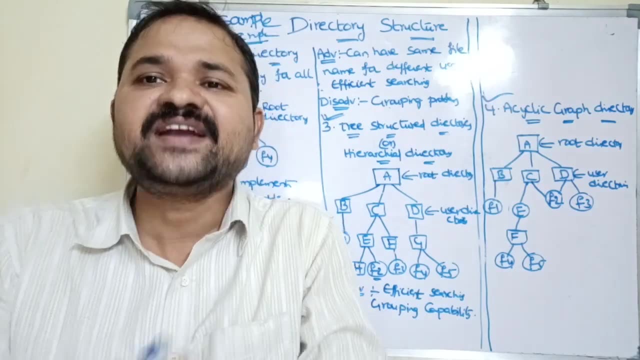 we'll use just the next approach. that is, nothing but this acyclic graph directory. acyclic graph directory is mainly useful if you want to share a file among different directories. so let's see this example here here. here we will share an approach and we might do a reasoned. 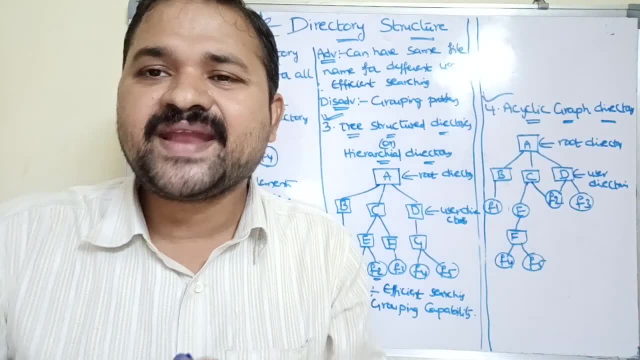 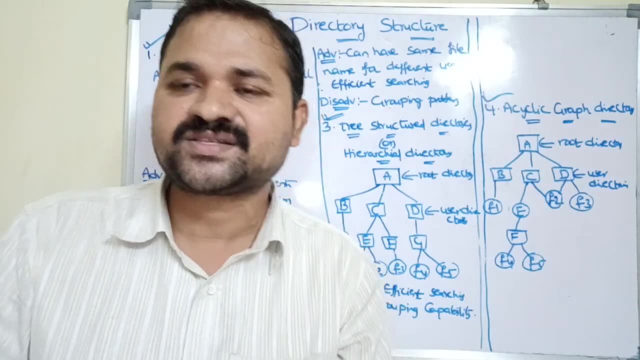 here we might do a reasoned. so here also we can have n number of directories. we can have more than two levels of directories. so level 0, level 1, level 2, level 3. so likewise we can have n number of levels, so we can create. 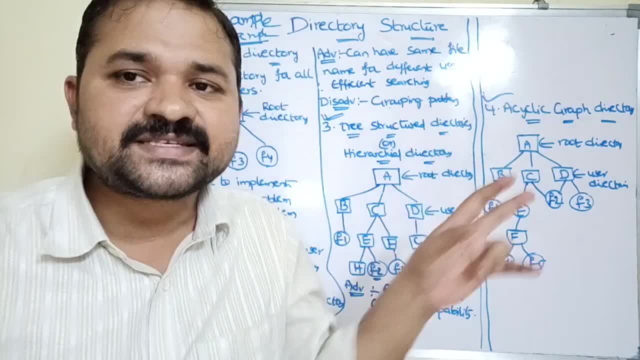 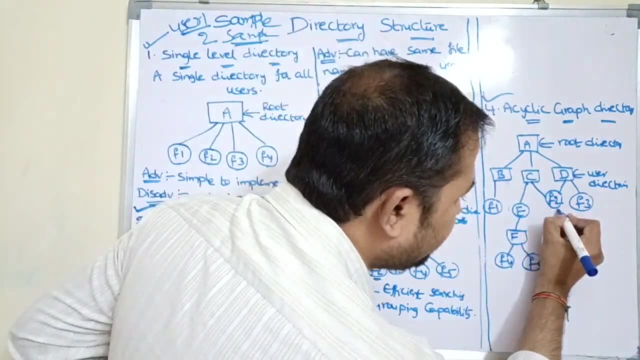 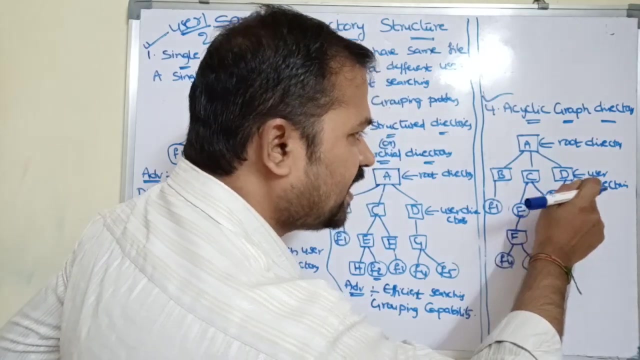 n number of sub directories, so it is our choice here. but acyclic graph directory means we can share the file among multiple directories. so let's take this example. so here we shared the file f2 among the directories c and d, so both c directory can use a cf2 file as well as d directory can use. 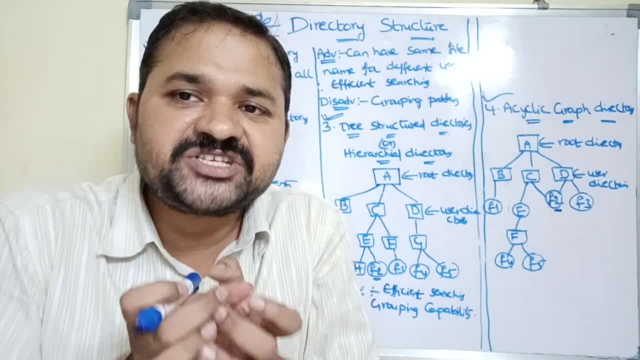 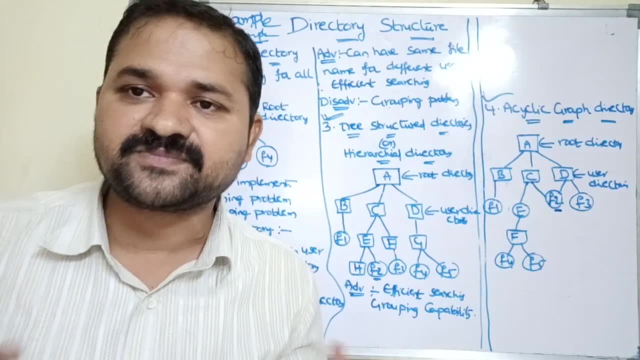 a cf2 file. so this is the advantage of this approach: so we can share a file between different directories. so this is about the directory structures which are available in the file system.